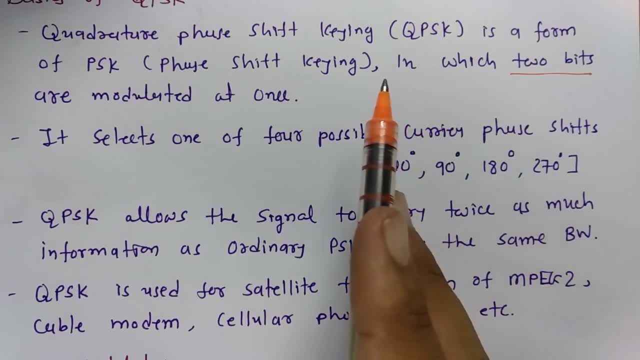 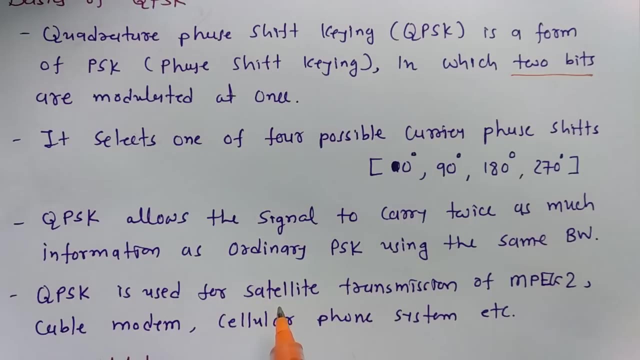 so qpsk basics is like: it is modulating two bits at once, it is having four different phase shifts, it is carrying twice information than bpsk with same bandwidth. and these are the applications where it has been utilized: in satellite transmission of mpeg-2, in cable model and in 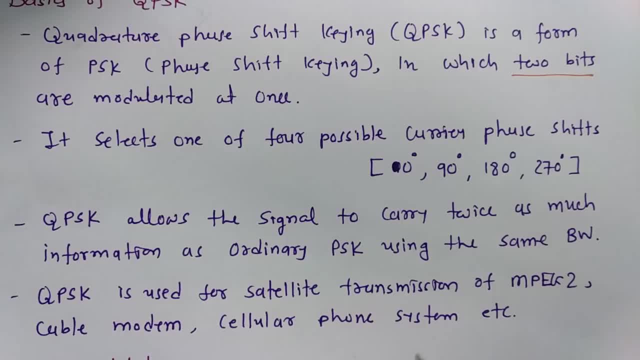 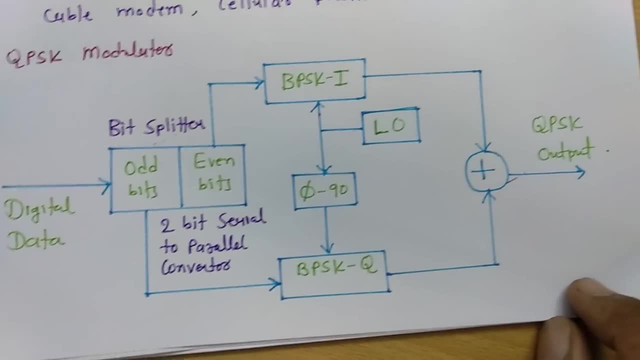 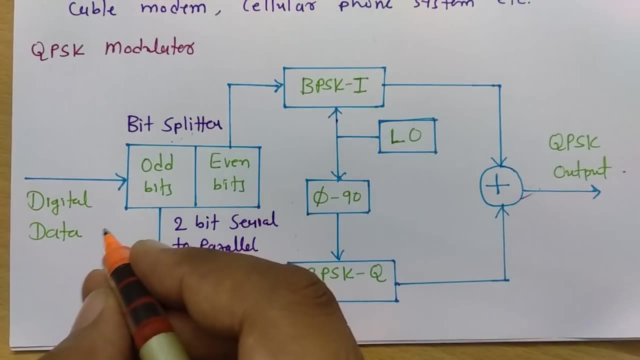 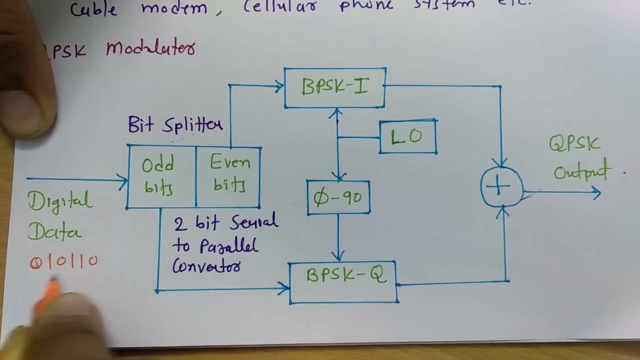 cellular phone system it has been utilized. so these are the basics which is there with qpsk. now let us move on to qpsk modulator. so one can see the basic block diagram of qpsk modulator, where here we have digital data. so it could be a serial digital data like 0, 1 0, 1 1 0. that is how. 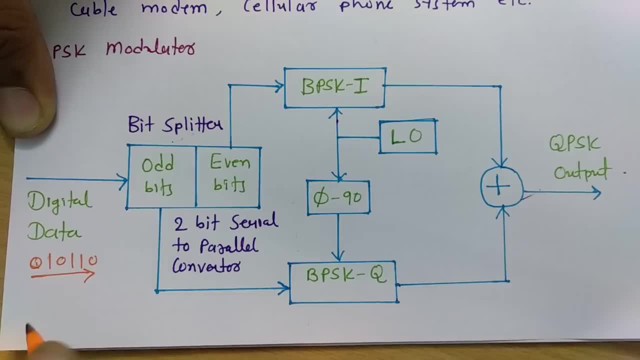 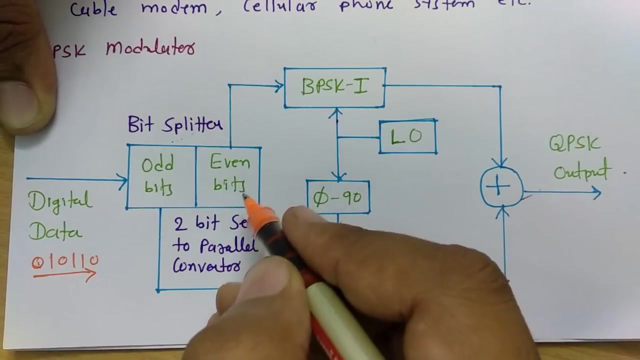 serial digital data that will be coming here now that will be given to bit splitter where even an odd bits that is getting split and it will come to bit splitter and it will come to bit splitter will convert this two bit serial to parallel data. So E1 data that will be coming over here and odd data that will be coming here. 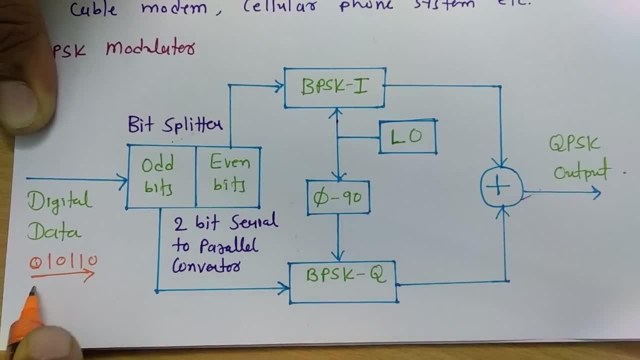 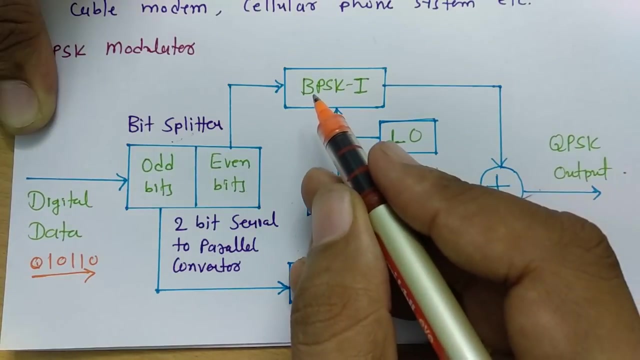 So if I say this is the bit stream, so E1 data stream that will be coming here out of this data bit stream and odd data bit stream that will be coming here, So E1 data bit stream that is being given to normal BPSK and let us say it is I channel. 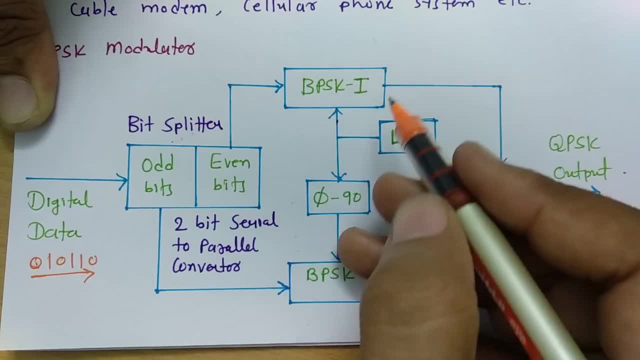 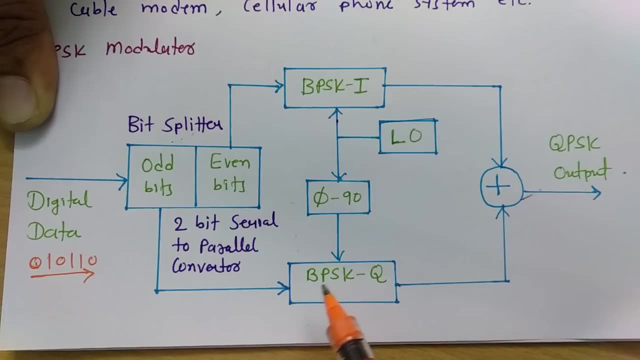 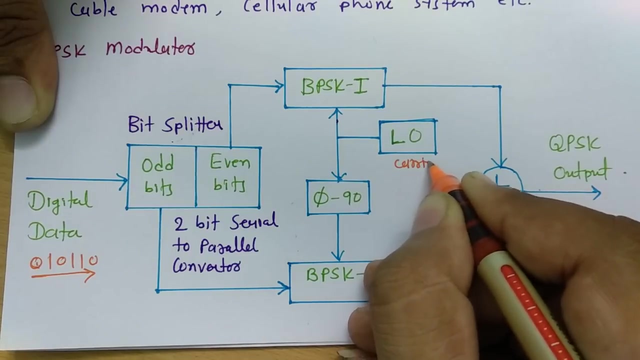 so BPSK I channel that will be coming here and odd data stream that is coming here and which will be given to BPSK Q channel. Now here we have local oscillator which is generating carrier, and that carrier that is directly given to I channel, BPSK. 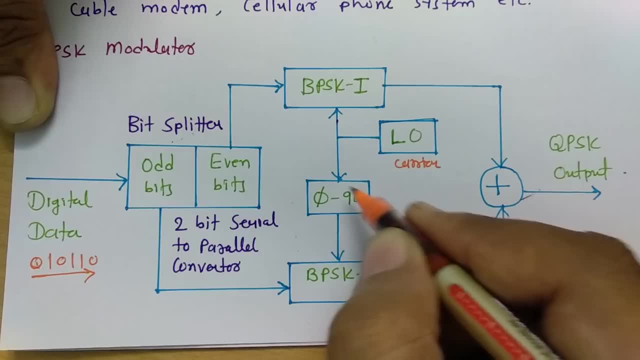 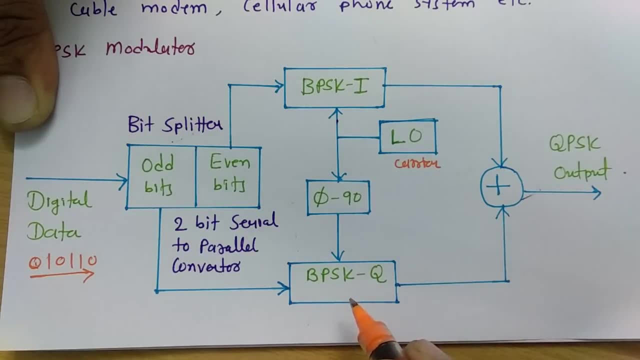 And that is being given to Q channel, BPSK with 90 degree phase shift. So here there will be 90 degree phase shift and it will be coming to Q channel. So ultimately, here you will be finding BPSK I channel and BPSK Q channel, with even an 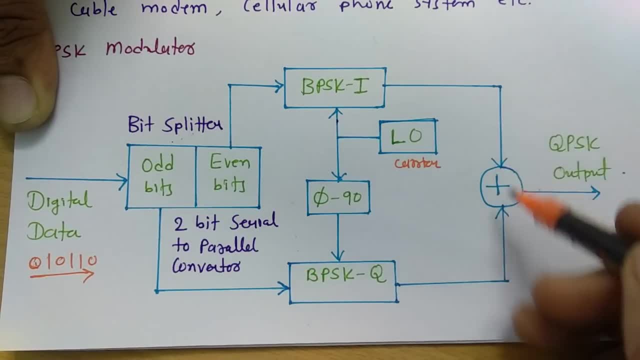 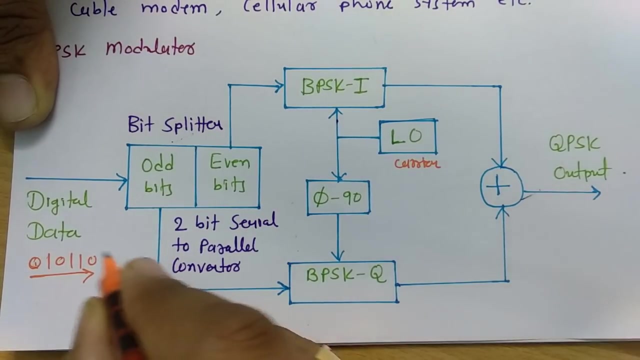 odd modulation and that is what we will be adding it over here, and that summation that will result into QPSK output, which is quadrature phase shifting output. Now what will happen here is here, if you have input data. so here we have serial data, but 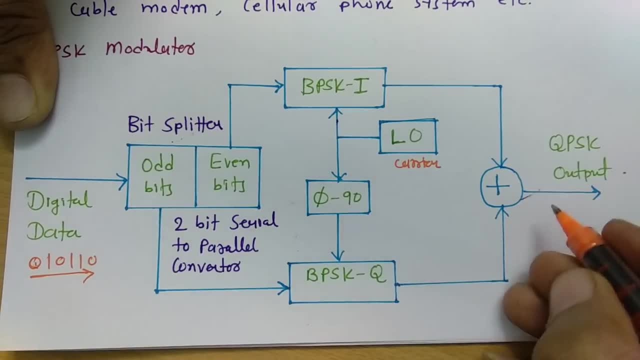 that is what we are translating into parallel. So if you have input data that is 0- 0, so in that case in carrier there will be 0 degree phase shift that you will be observing in QPSK If your input data that is 0- 1.. 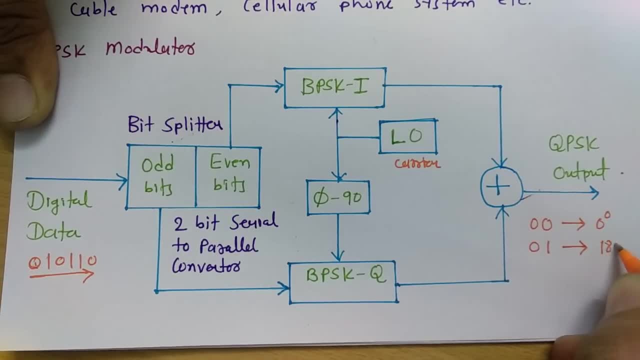 So in that case you will be observing phase shift. Phase shift that is 180 degree If your input data that is 1: 0.. So in that case here phase shift is 90 degree and if your input data that is 1: 1.. 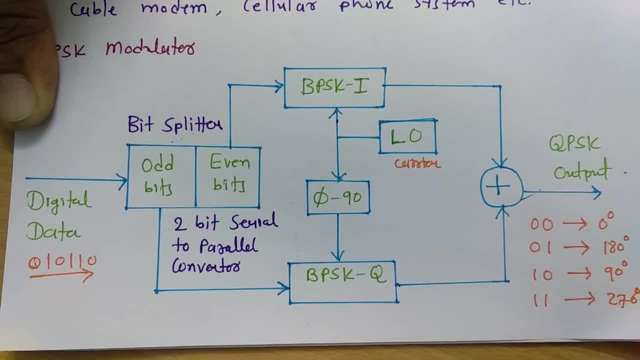 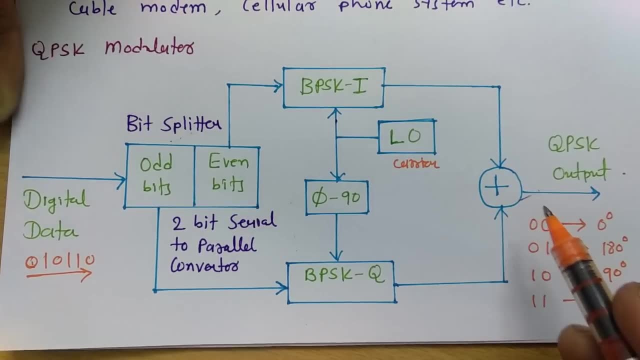 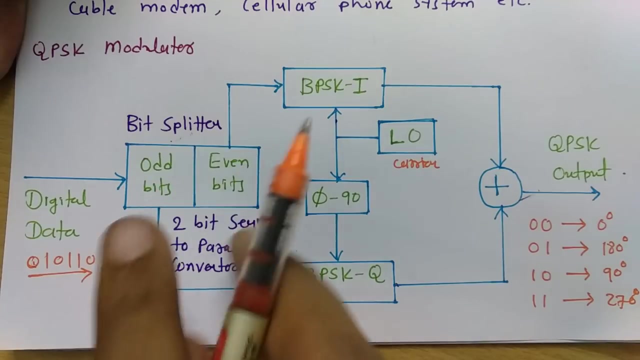 In that case here phase shift is 270 degree, So output phase that is varying with respect to input bits. So in QPSK there are two bits. that is what we are modulating at once. So here two bits that is going in this and that is getting splitted into even and odd. 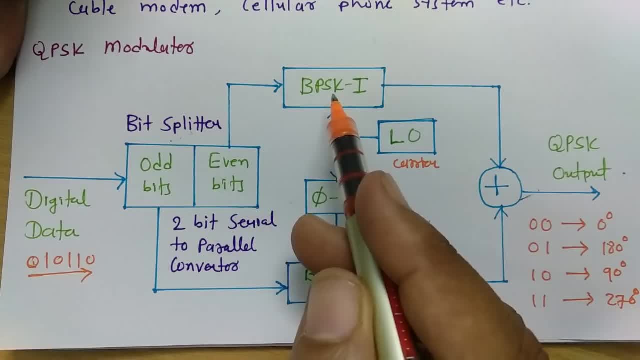 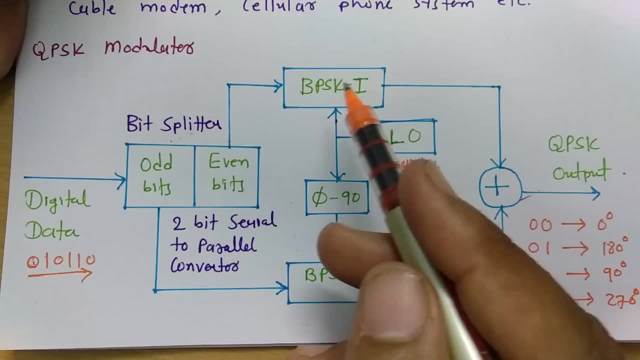 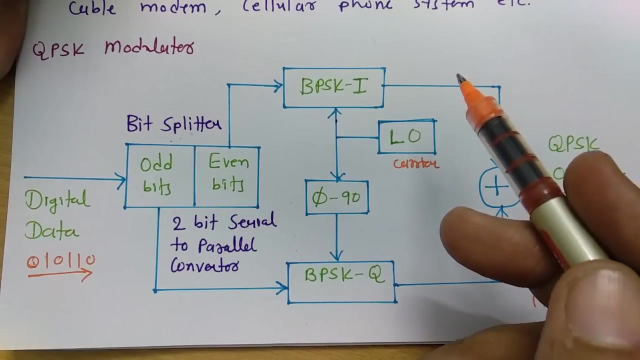 bits. even that is being given to BPSK I and odd that is being given to BPSK Q and both is having carrier- I is having direct carrier and Q is having 90 degree shifted carrier- and that is what getting modulated here and added will result into QPSK output. 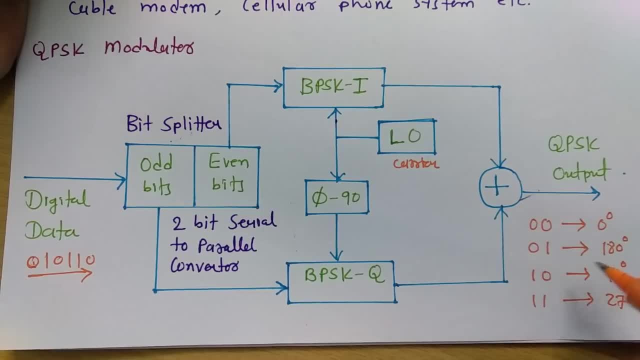 So. So here, two bits will have 0 phase shift, 0, 1 will be having 180 degree phase shift, 1, 0 will be having 90 degree phase shift and 1: 1 will be having 270 degree phase shift. So let us try to understand how waveforms will appear. 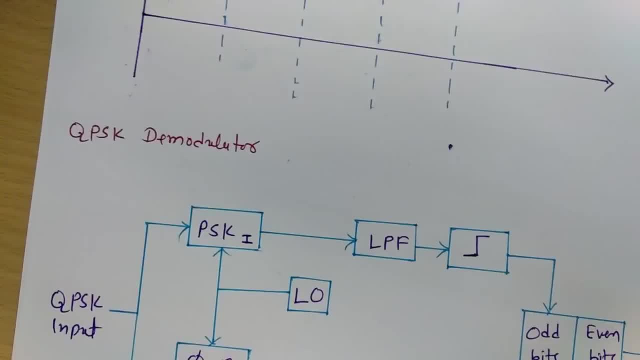 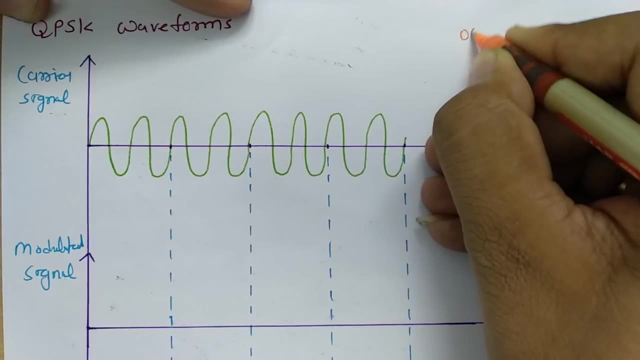 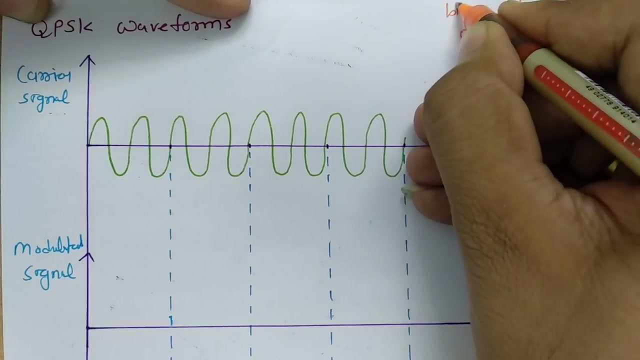 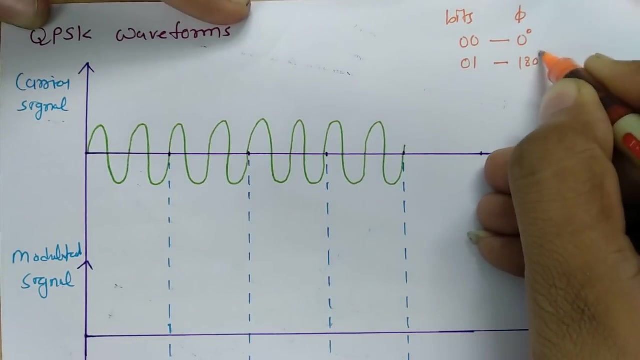 So that will give you a clear idea about how QPSK is working. So here to understand waveforms: as I have told, if you have input data that is 0- 0. So that will result into 0 degree phase shift. And if your bits are 0- 1, in that case phase shift is 180 degree. if it is 1- 0, in that case. 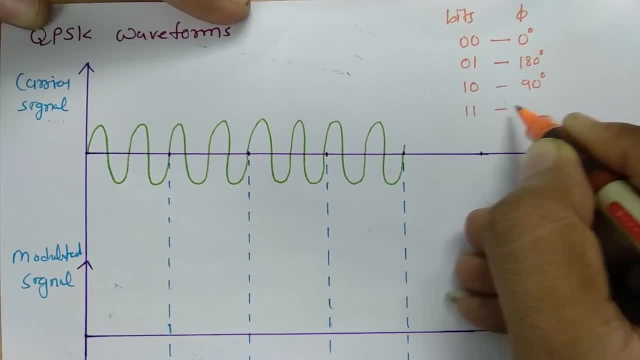 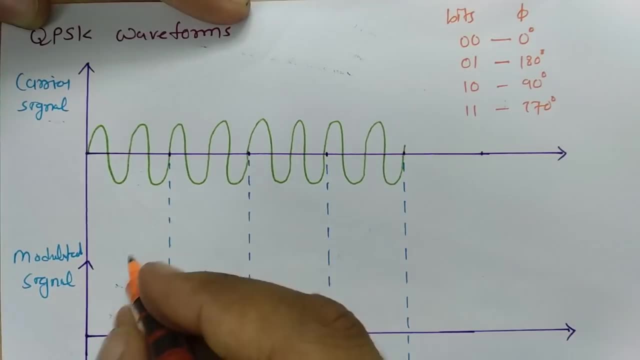 phase shift is 90 degree, and if it is 1, 1, in that case phase shift is 270 degree. So here we have a carrier signal. one can see if I say my bits are 0, 0 right over here, if I say my bits are 0, 1.. 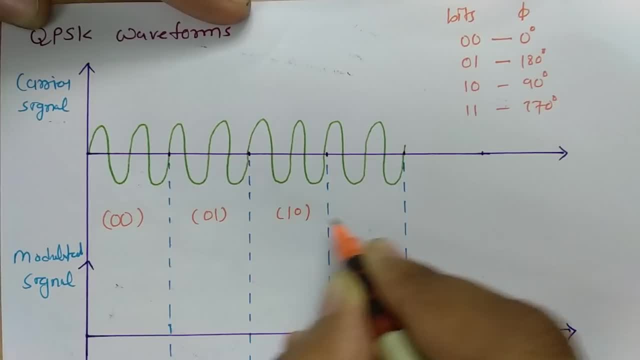 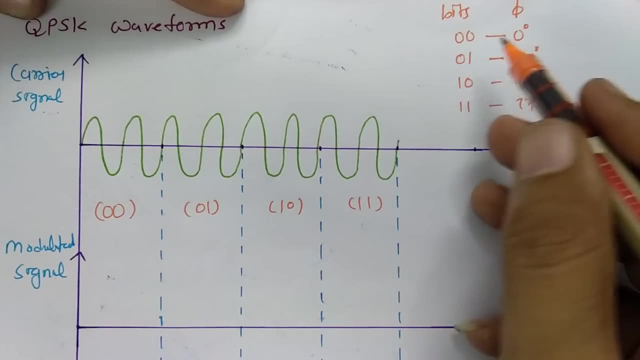 Right Here my bits are 1: 0 and here my bits are 1: 1.. So what will be my modulated signal? So for 0: 0, phase shift is 0.. So this is what carrier, without having any phase shift, you will be getting that modulated. 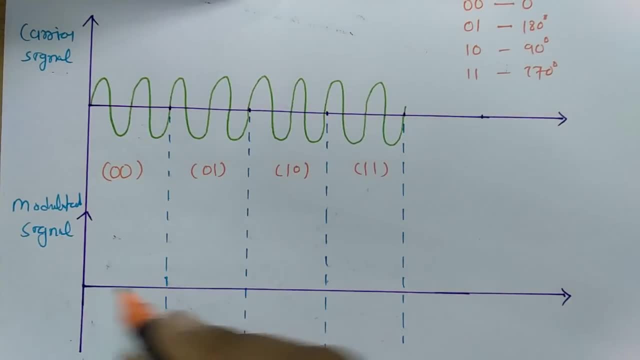 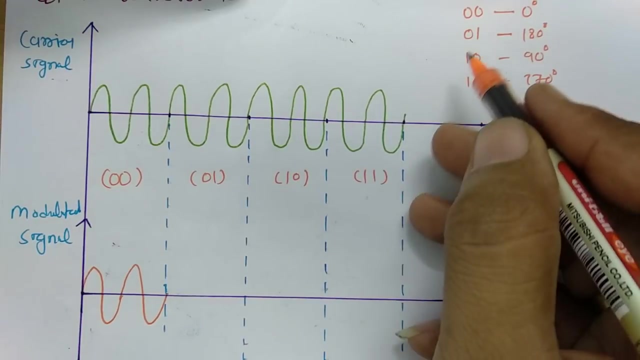 signal. So with 0 phase shift you will be getting modulated signal. So that is as similar as this signal one can see. So with 0 phase shift, 0- 0. That is getting modulated If bit is 0- 1. if two bits are 0- 1, in that case 180 degree phase shift is there. 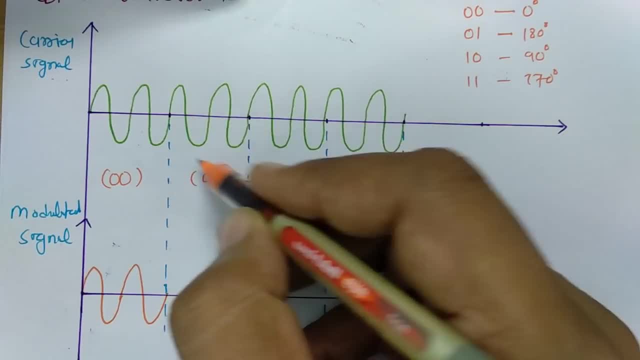 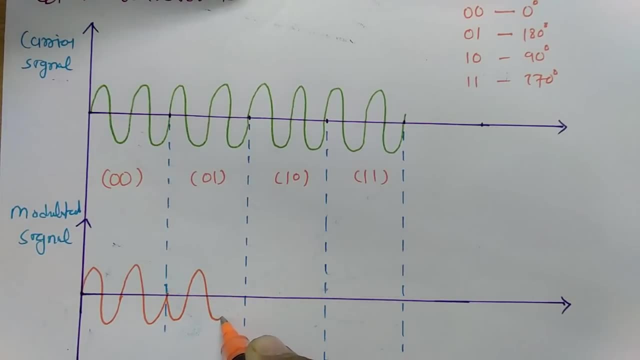 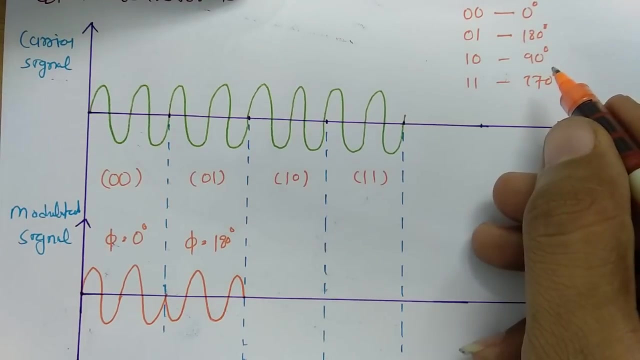 So you can see carrier signal is like this. So 180 degree shifted version will be this. So here you can see, phase is 0 degree shifted and here phase is 180 degree shifted. Now, if bits are 1- 0, in that case 90 degree phase shift is there. 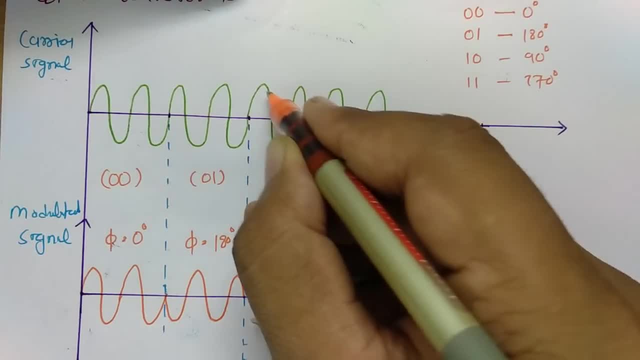 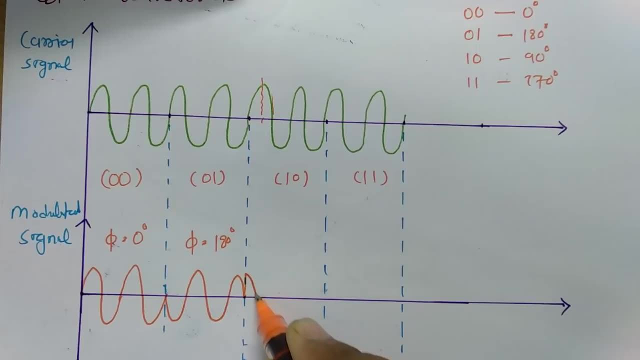 So for 90 degree phase shift, signal will initiate from here with 90 degree phase shift. So you will be finding signal that will initiate from here. And for 1: 1. Phase shift will be 270.. Here phase shift was 90 degree. 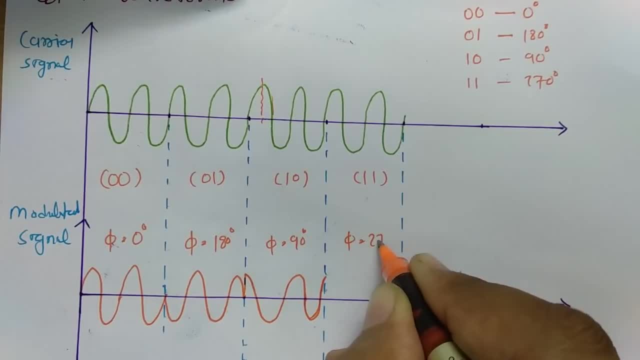 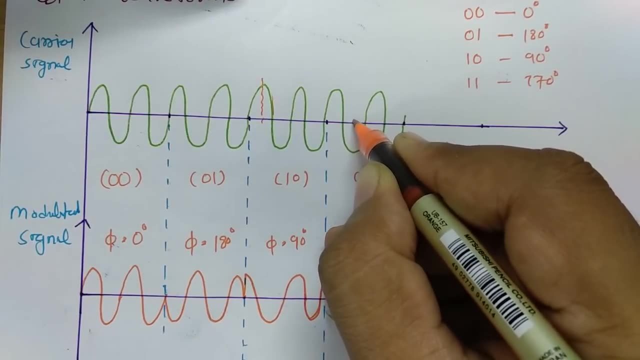 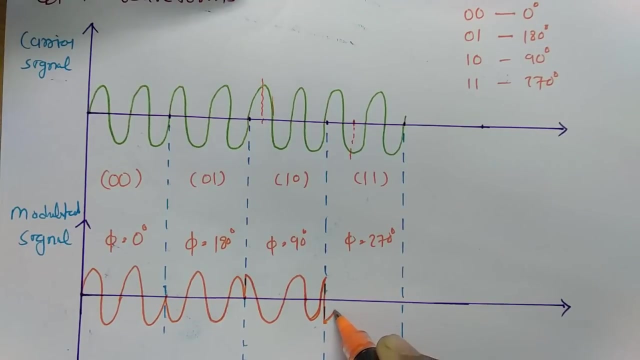 For 1: 1 phase shift is 270 degree. So here phase shift will be 270 degree. So at 270 degree, this is 180 and this is 270.. So signal will start from here. It means you will be finding signal starts from here. 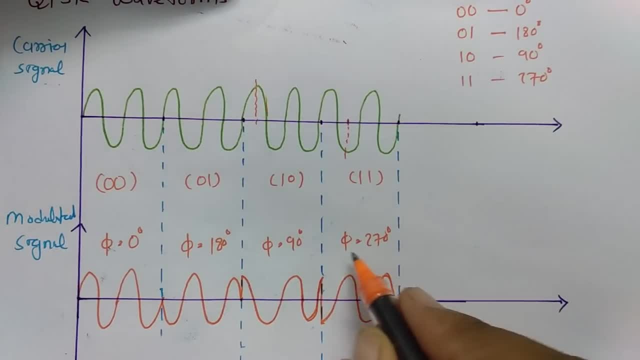 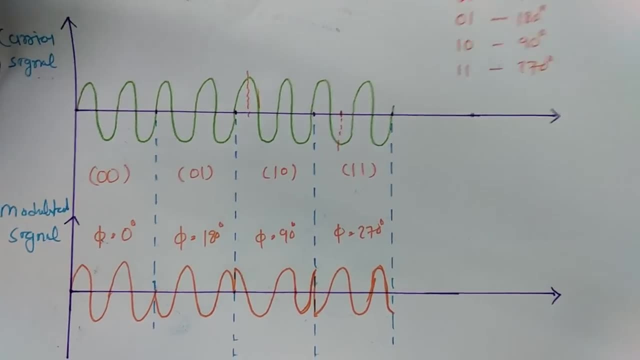 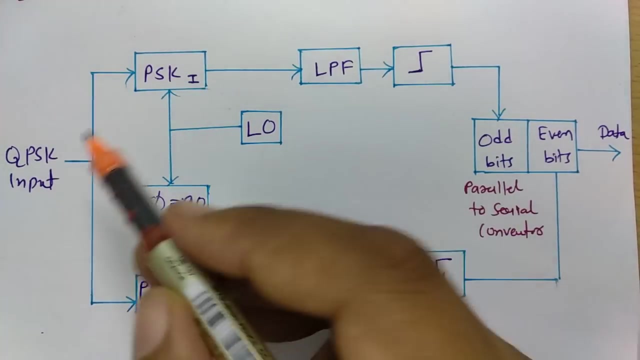 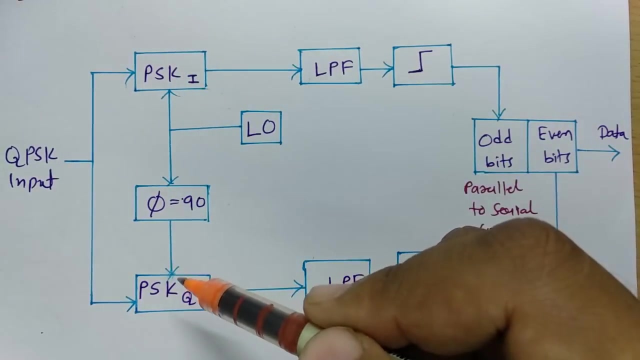 So phase shift over here. that is 270 degree. So that is how waveforms will appear for QPSK. Now let us try to understand demodulation process. So in demodulation process here we have QPSK input. Now that QPSK input that is been given to PSK demodulator with I channel and Q channel. 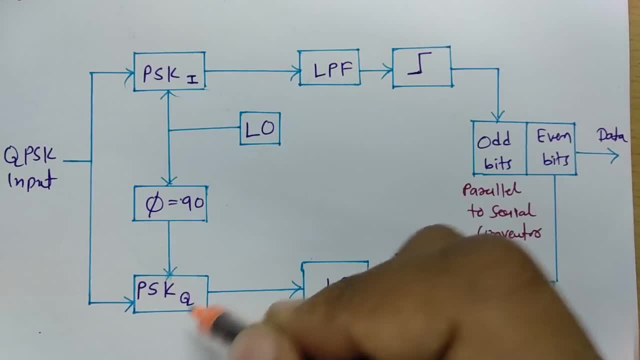 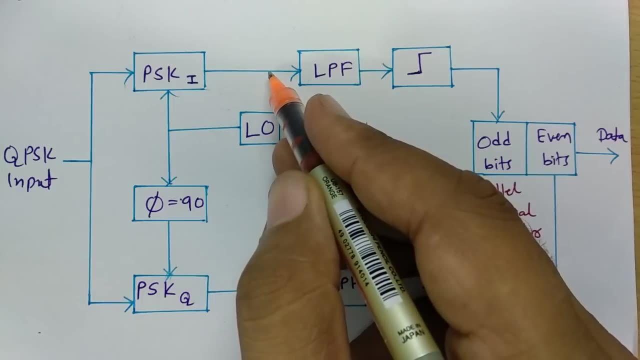 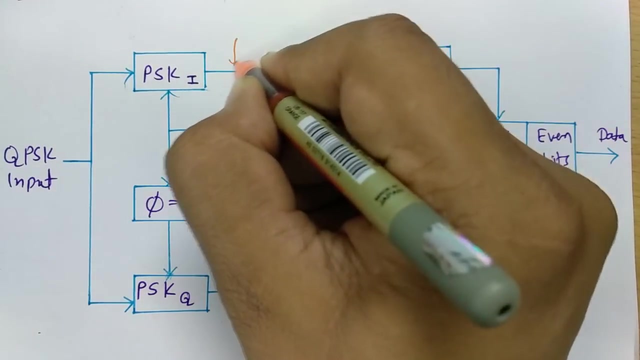 In I channel carrier is directly given And in Q channel Carrier is given with 90 degree shifted version. So here you will be getting demodulated I channel And here you will be getting demodulated Q channel. So here you will be having demodulated I channel. 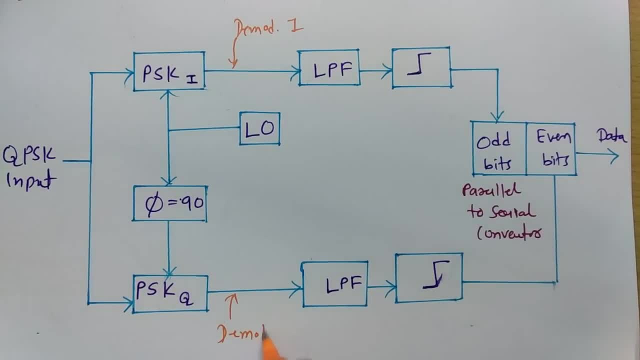 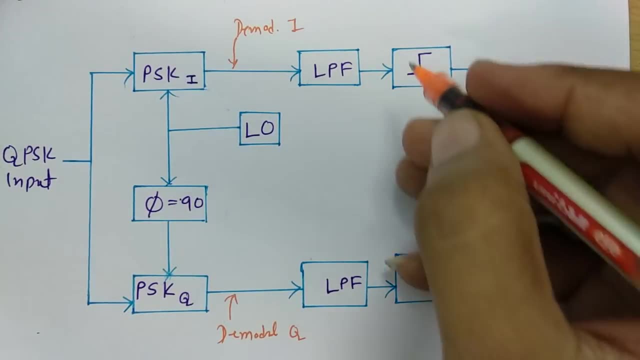 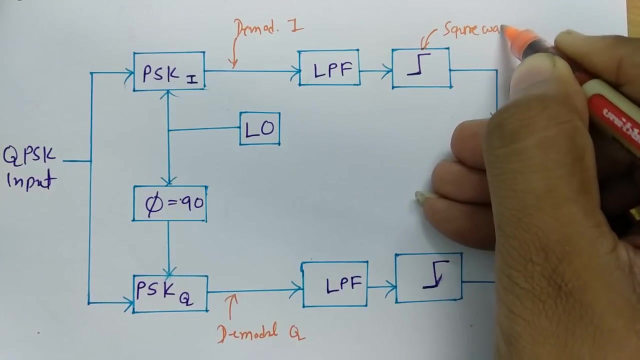 And here you will be getting demodulated Q channel, And that is what we are: passing it through low pass filter And then it will be given to square wave generator. So this is square wave generator. So what will happen is like: now you will be getting this signal in terms of digital data. 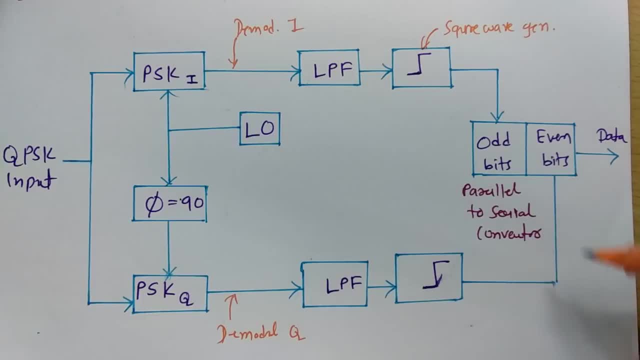 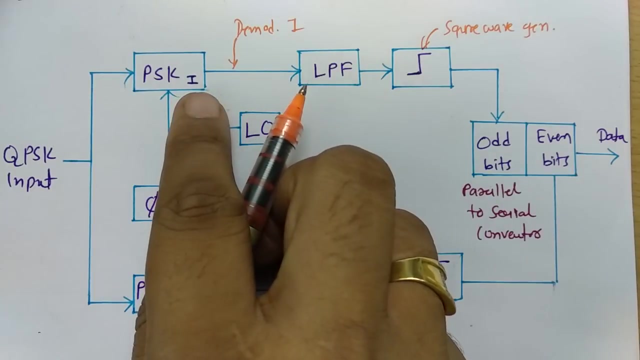 And that digital data is having odd bits over here and even bits over here. So this parallel data that we are translating into serial by having this block. So this is what We are generating: parallel data to serial data. So odd bits that is been generated by PSK demodulator and even bits that is been demodulated. 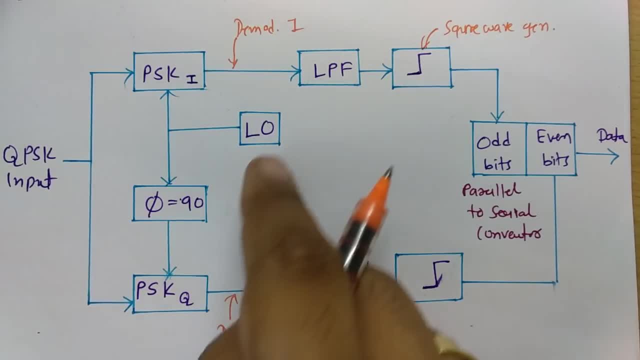 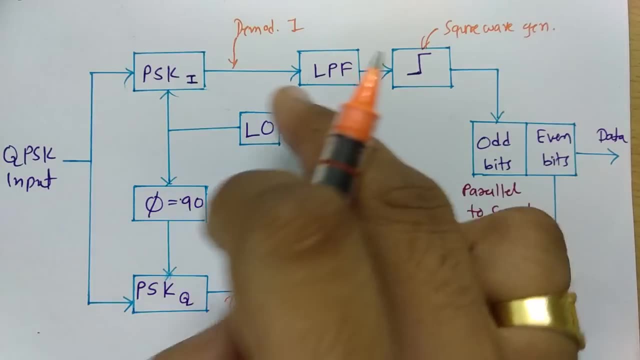 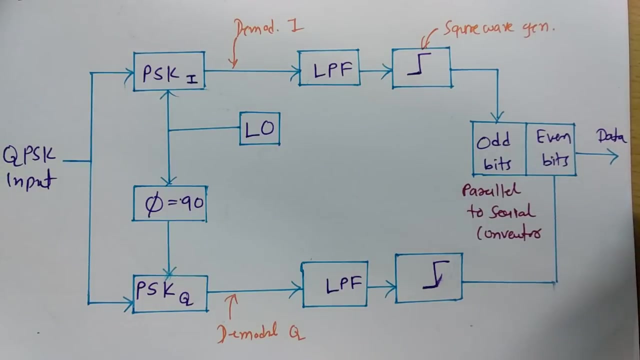 by PSK Q channel, But Q channel that is having carrier with 90 degree phase shift and I channel that is having carrier with zero degree phase shift. And this, two parallel bits, that is been converted into serial and that is what our original data. 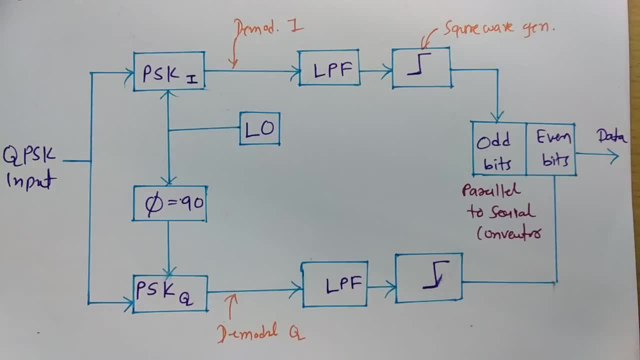 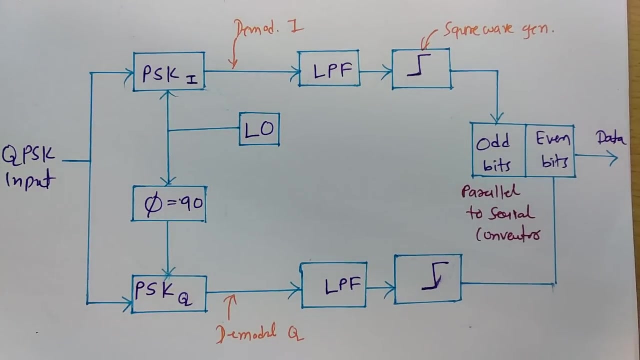 So that is how we have QPSK demodulation process. I hope that you have understood this. You can ask your queries in comments. definitely, I will get back to you And if you have any doubt, you can place that in comment section. definitely will be having. 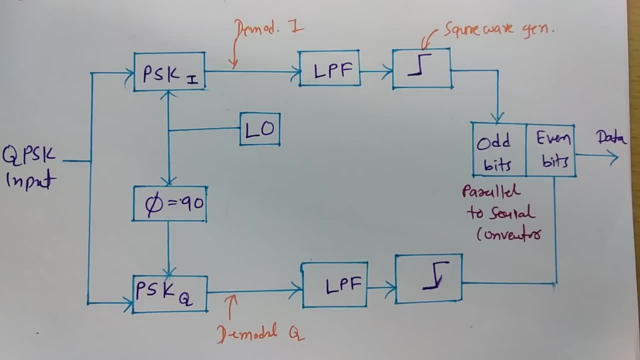 discussion and in future I will place videos to sort out all those queries and that will be beneficial to students. Thank you so much for watching this video.